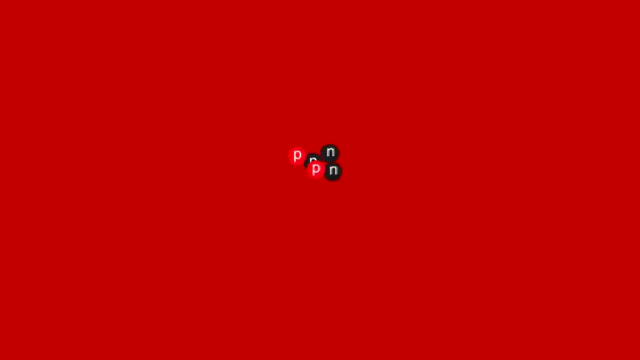 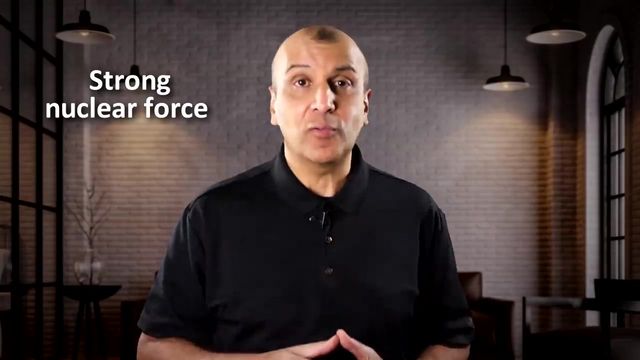 what keeps them glued together so tightly? Well, it turns out that the force keeping them together is even stronger than electromagnetism. In fact, it is about 100 times stronger. It is the strongest force in the universe, And physicists creatively call this force the strong nuclear force. 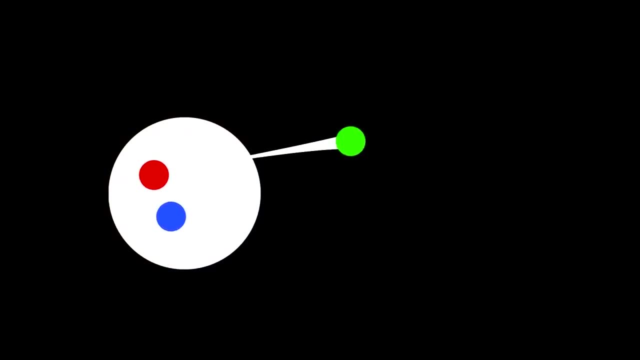 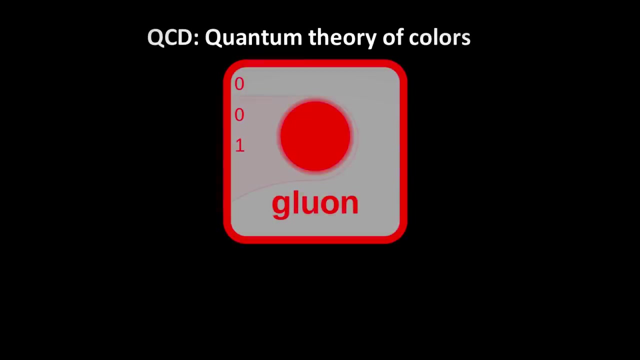 And amazingly we, A brained humans, happen to have figured out how this force works pretty darn well. It's really strong, but works only at very short distances, And it's also a very colorful force. That's why its study is called quantum chromodynamics, In other words, 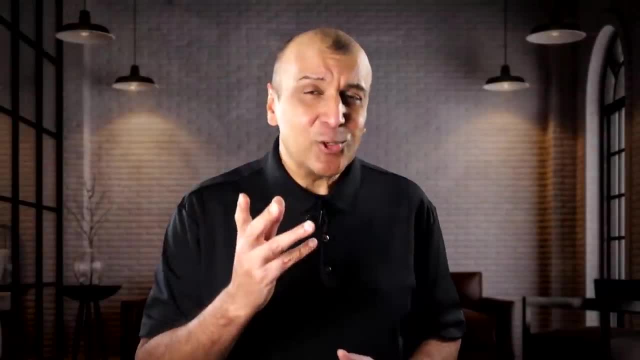 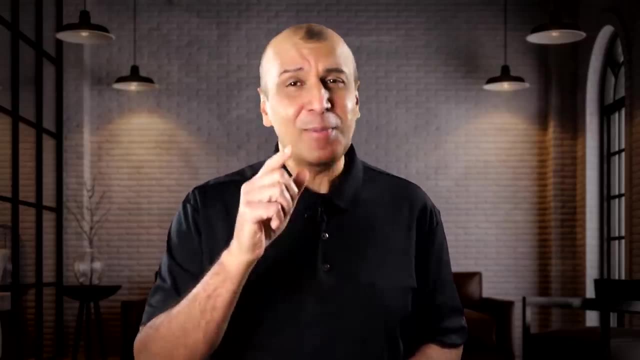 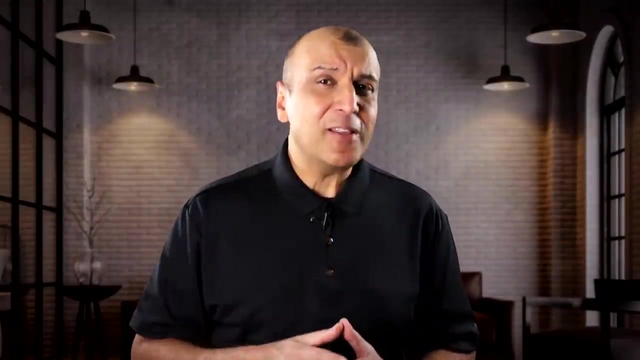 it's the quantum theory of colors, But, as you'll see shortly, these are not the kind of colors you're used to seeing. What the heck am I talking about? That's coming up right now Before we talk about the fascinating science of the strong force. I'd like to thank today's sponsor. 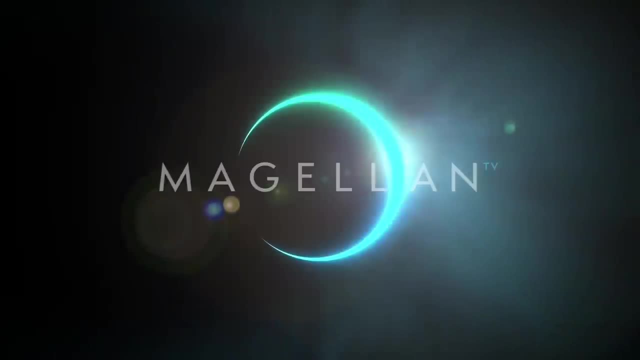 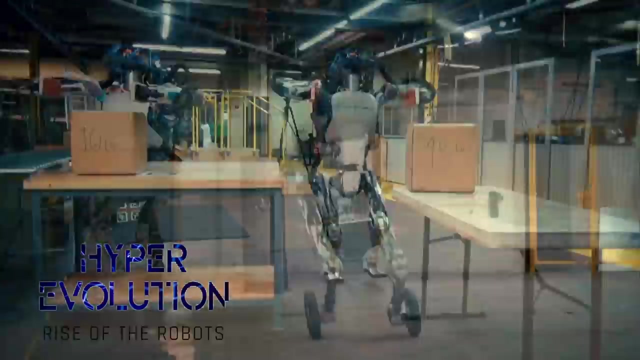 Magellan TV for making this episode possible. Magellan is an ad-free documentary streaming service created by documentary filmmakers. Their collections are richer and broader than just about any other streaming service around. You can dive deep into subjects like history, culture and of. 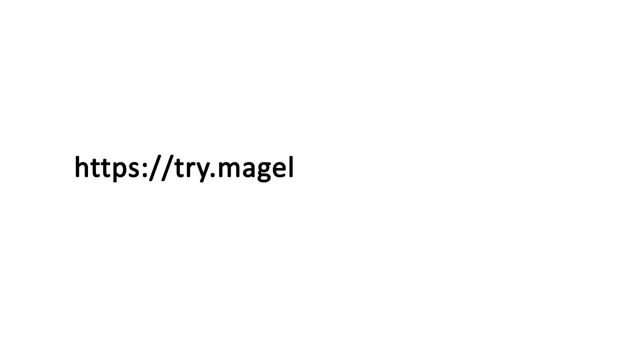 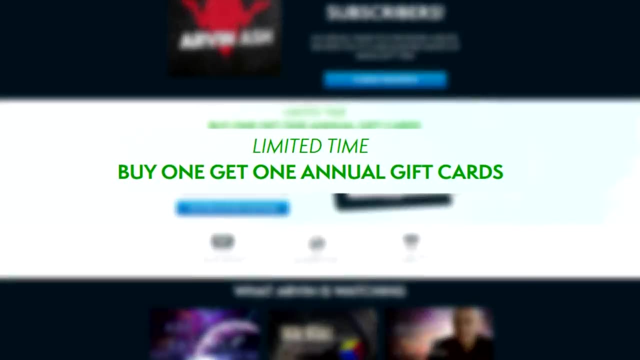 course, science. You can learn more about the science of the strong force in this episode. I'm excited to tell you that Magellan is offering a buy one, get one free gift card for the people in your life that you want to give the gift of knowledge. Click the link in the description. 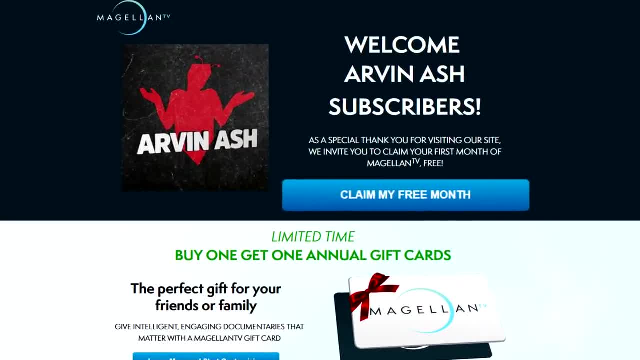 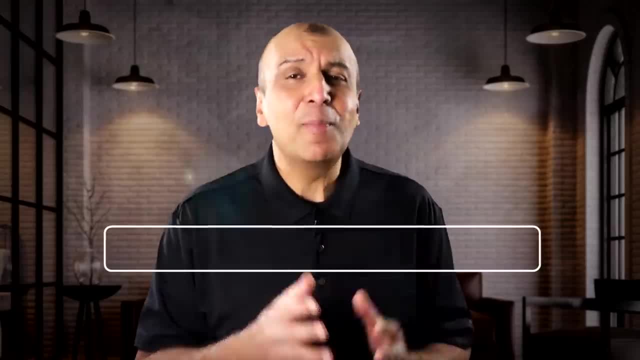 to take advantage of this. If you're new, you'll get a free one-month trial of Magellan. If you're already a member, you'll get an extra month any time you purchase a gift card. There has never been a better time to spread the gift of knowledge. I highly recommend Magellan TV. 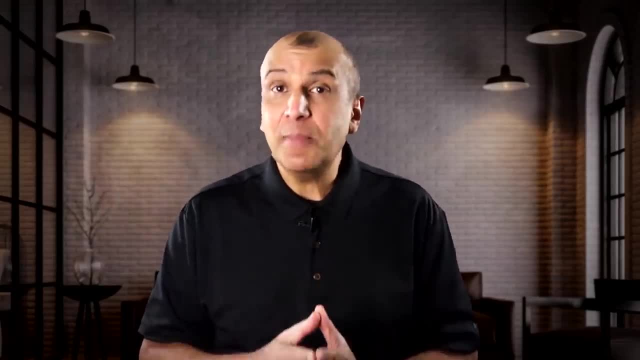 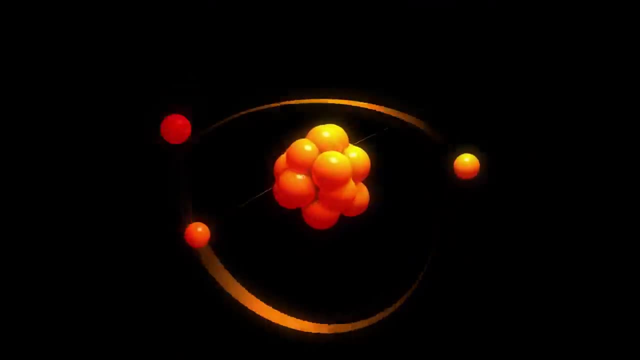 so be sure to click the link in the description. In the 1920s, it became clear that the atom was made up of negatively charged electrons and a positively charged nucleus. This model, although great in its simplicity, left one big question: If, like charges repel each other. 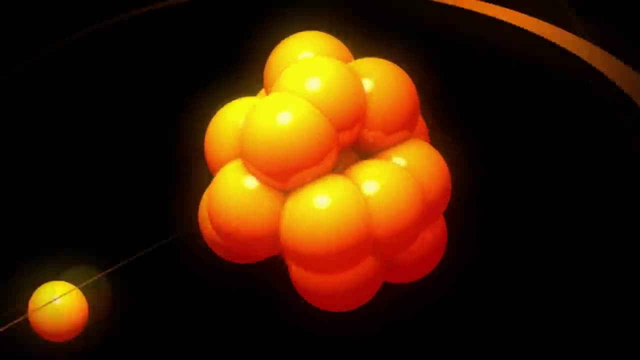 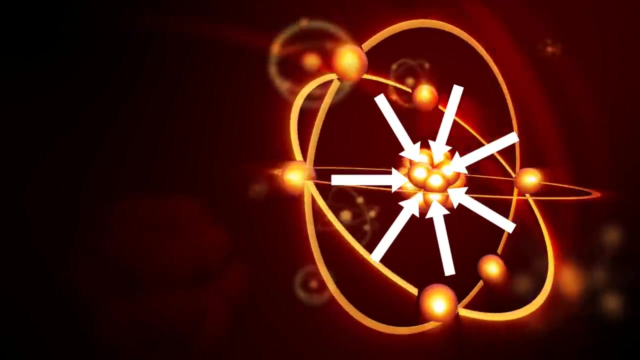 how can you pack positive protons so close together in the nucleus? It was obvious that there must be some extremely strong force which can overcome this repulsion. One of the great minds that sought to answer this question was Japanese physicist and later Nobel laureate. 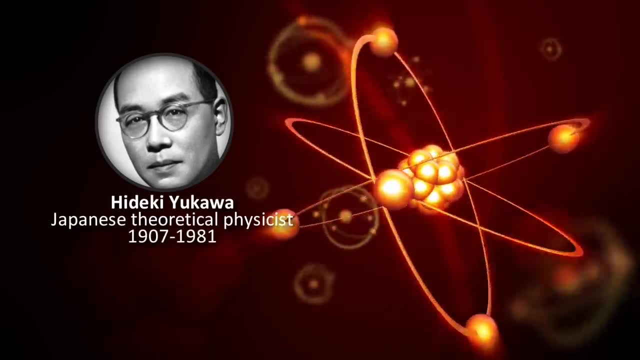 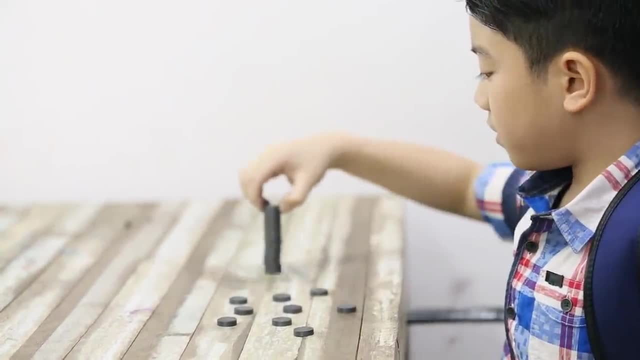 Hideki Yukawa. He proposed the idea that the atom was made up of negative charged electrons and a positive charge repel each other. He proposed the first significant theory of this strong force in 1934.. He realized that since electromagnetic repulsion happens on large scales, for example, 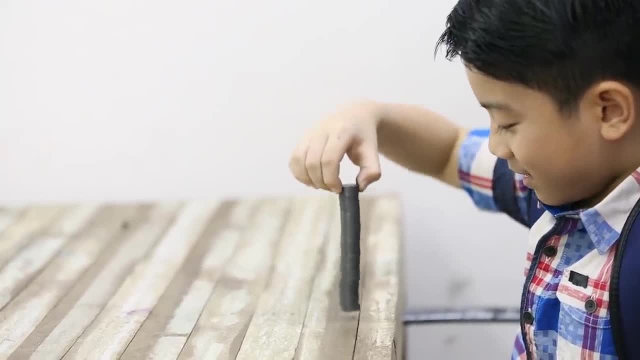 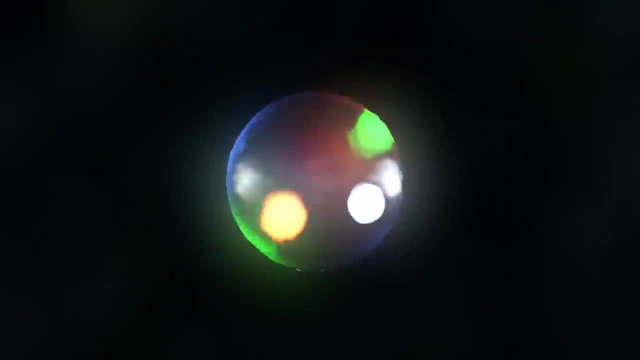 we can see its effects in our macro scale world when playing with magnets. this strong force, which opposes electromagnetic repulsion, must occur on a very small range because we don't see the effect of this strong force in our macro world. Another clue that the range of 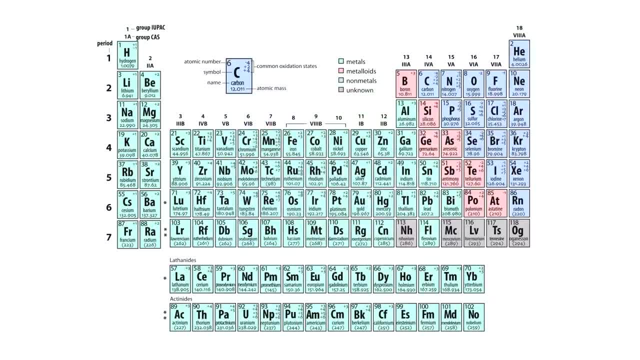 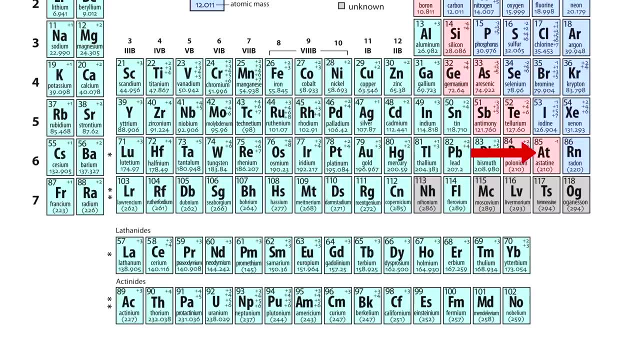 this force has to be small is because there appears to be a maximum size of atomic nuclei. Any nucleus larger than the size of a lead nucleus is unstable, suggesting that there is a point beyond which the strong nuclear force can't hold the nucleus together. 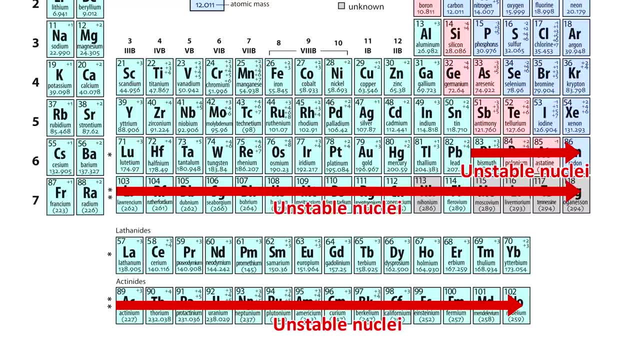 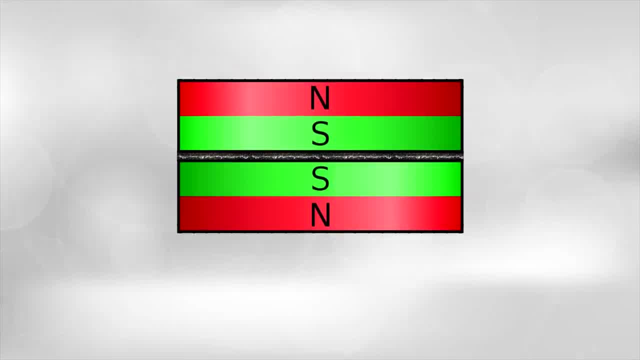 This also suggests that the range of the force must be smaller than an atom. The analogy is like Velcro: If you put Velcro on two similar poles of a magnet, if they are close enough the Velcro will overcome the repulsion and keep them together. But if the 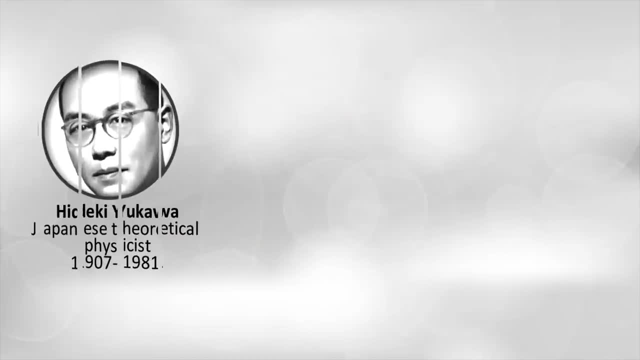 magnets are not touching the Velcro makes no difference. Yukawa proposed that there must be a massive mediator particle that transfers this force between protons and neutrons. Using Einstein's energy equivalence principle equals mc squared and Heisenberg's uncertainty principle, which says that the uncertainty in energy times the uncertainty in time. 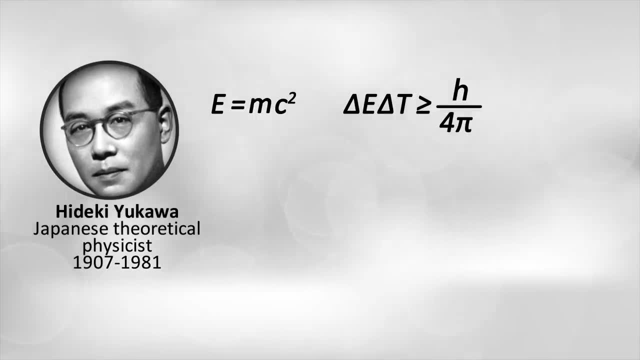 is greater than or equal to h over 4 pi. he solved the equation to find an approximate mass. The range of this force can be found by multiplying c, the speed of light times the time of the particle's existence. Time, therefore, is just. 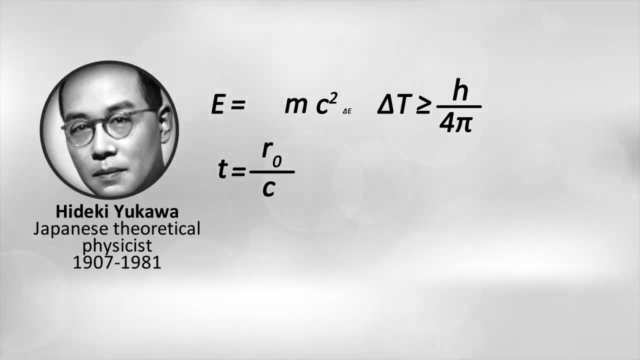 the range divided by c, We can set the range r knot as just the radius of the nucleus. Then by knowing the time, we can find the energy or mass. Plugging in the numbers we get a mass of about 100 mega electron volts or MeV. 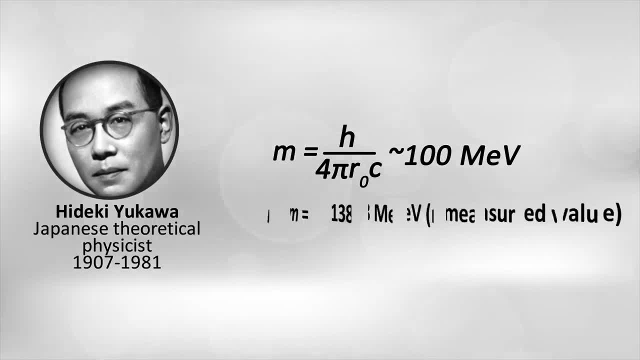 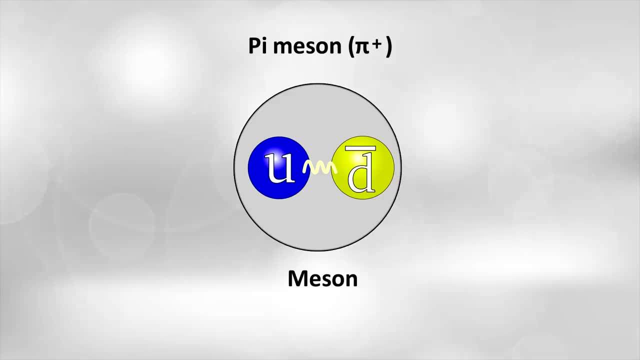 And this is remarkably close to what was found later to be the correct answer, which was about 138 MeV. Yukawa coined the term meson to describe this particle. Meson means middleweight: The leptons, like electrons, are lightweight, and baryons, like protons and neutrons. 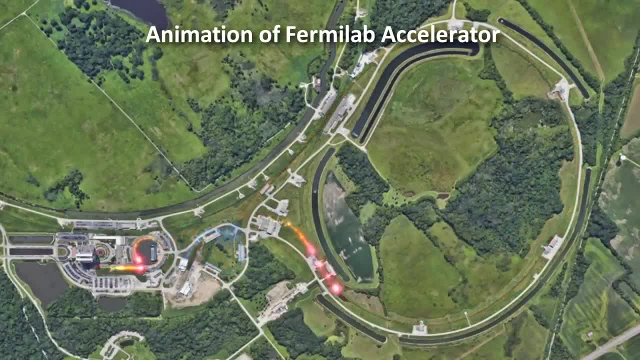 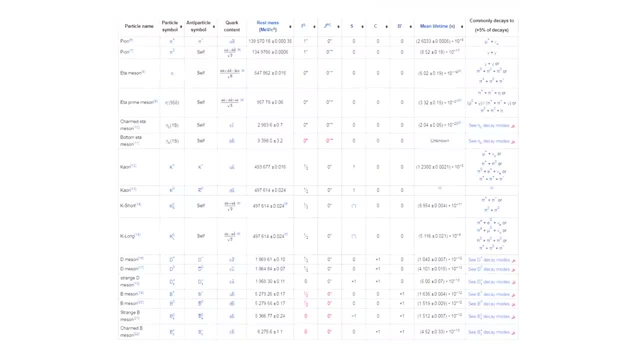 are heavier. Anyway, as more experiments were being done in particle accelerators, new mesons and other types of particles kept getting discovered, dozens in fact. This created a kind of crisis in particle physics, because it was not thought that these particles could all be fundamental. 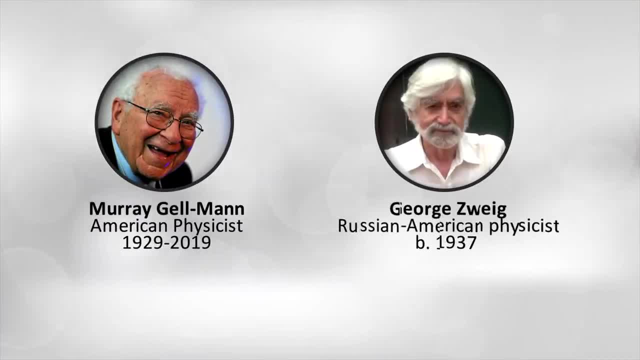 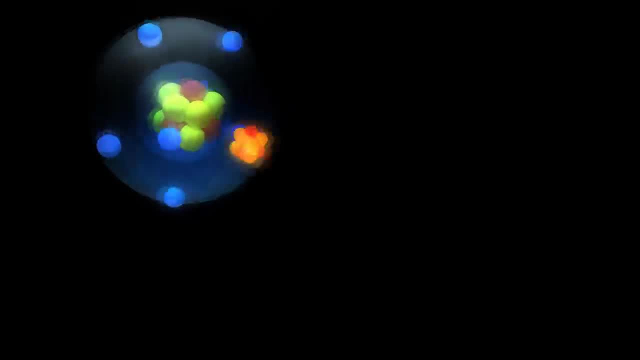 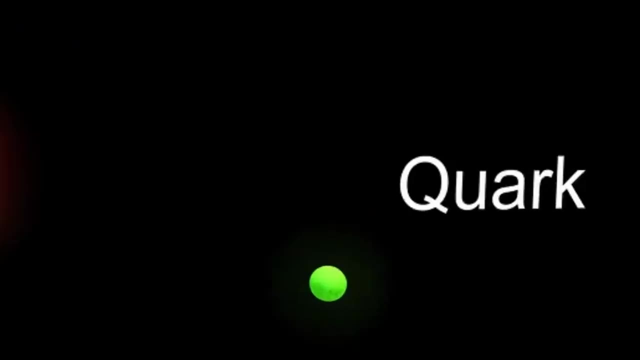 In 1964, Murray Gell-Mann and George Zweig proposed that the various mesons and other particles that interacted with the strong nuclear force could be explained if they were composed of even smaller but fundamental particles. Gell-Mann called these particles quarks, from a term in a novel by Irish author. 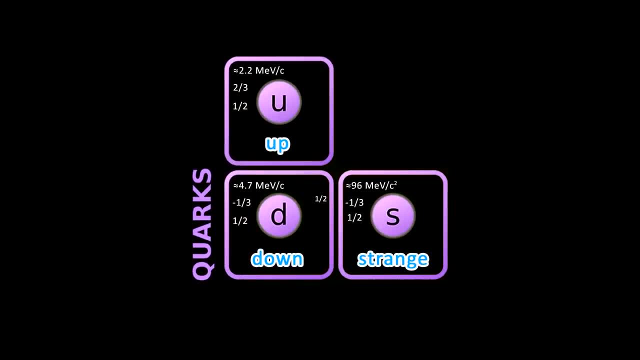 James Joyce Gell-Mann proposed that there were three types of quarks, now called up down and strange. The up quark has a charge of two thirds, whereas down and strange have a charge of negative one third. All had a spin of one half and they all experienced a strong force. 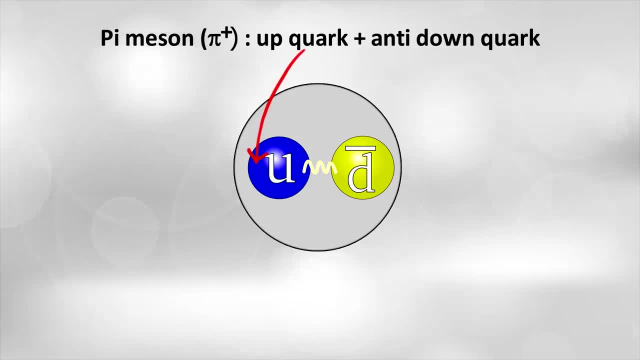 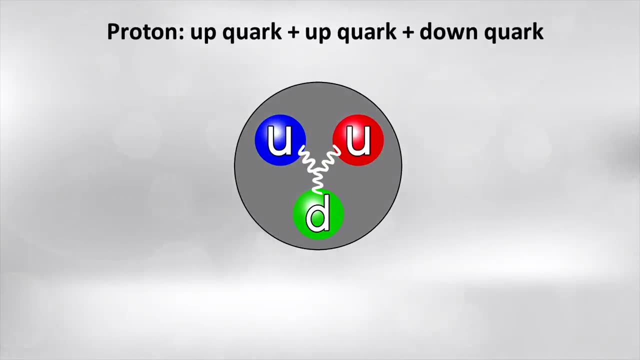 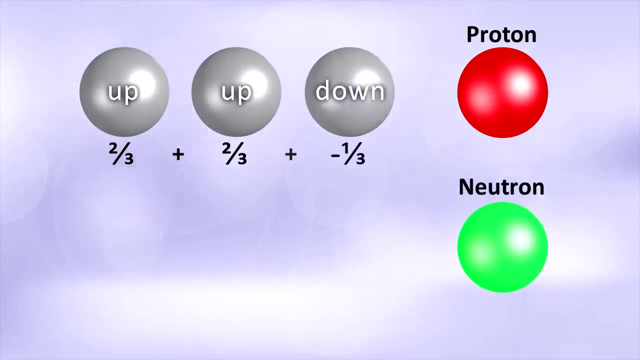 The quark model proposed that mesons were made up of quark-anti-quark pairs, But another way these quarks could combine is in groups of three quarks. These became baryons or heavy particles such as protons and neutrons. A proton is made of two up quarks and a down quark. You'll notice. 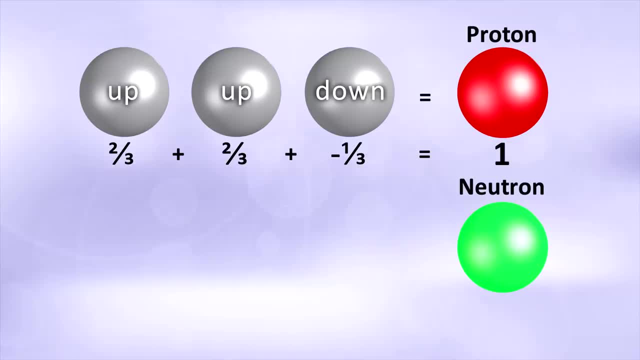 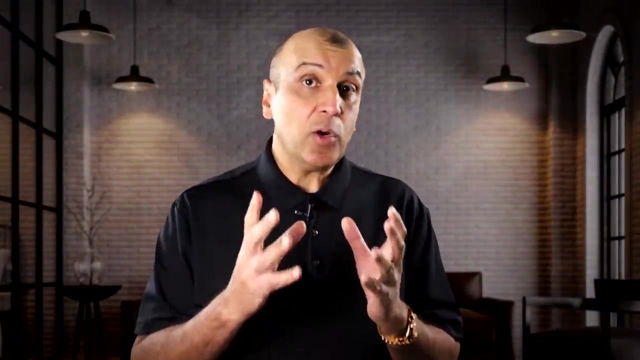 that these charges add up to plus one. The neutron is composed of two down quarks and one up quark. You'll notice that the charges add up to zero. Other combinations of these quarks form the other heavy baryons, But this had a major problem, and that is the idea of having three. 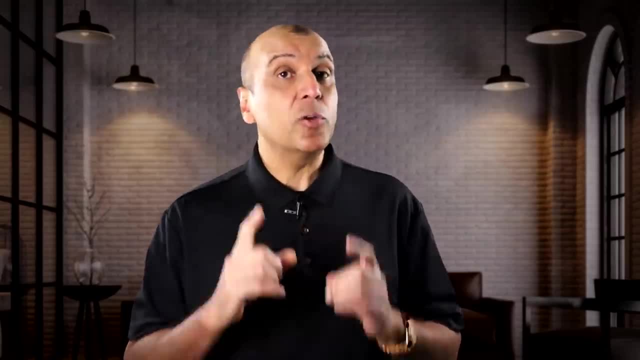 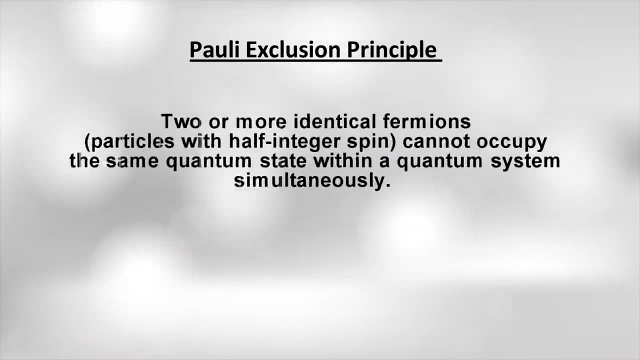 up quarks within the same particles. This, according to quantum mechanics, should be impossible because at least two of them would have the same quantum properties And, according to the Pauli exclusion principle, two fermions like quarks with the same quantum properties cannot exist in the same location at the same time. 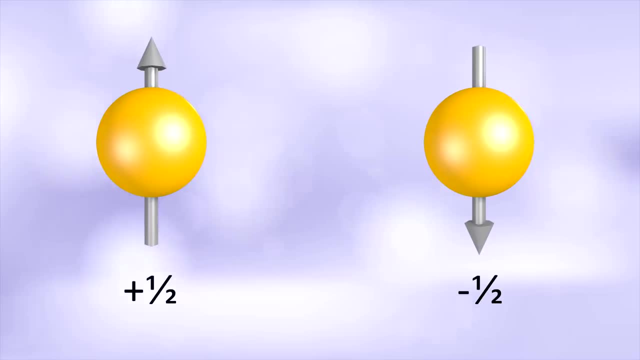 This principle is the reason you can have only two electrons in any atomic orbital, because the electrons can have a spin of either plus one half or minus one half spin. If you put three or more in the same orbital, it would have to have a spin identical to one of the already existing. 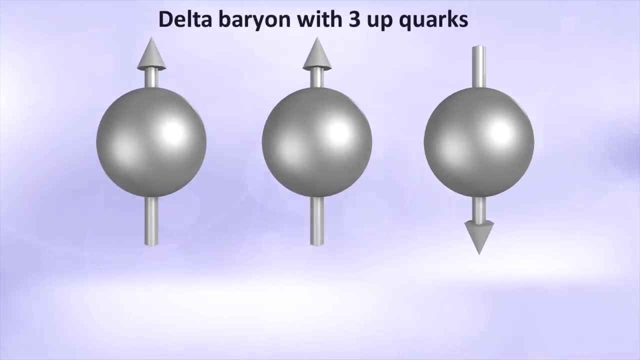 electrons in that orbital. But one of the detected particles, called a delta particle, was composed of three of the same quarks, up up and up, for example. In that case, since these particles all have a spin of one half, we can have one particle that is spin plus one. 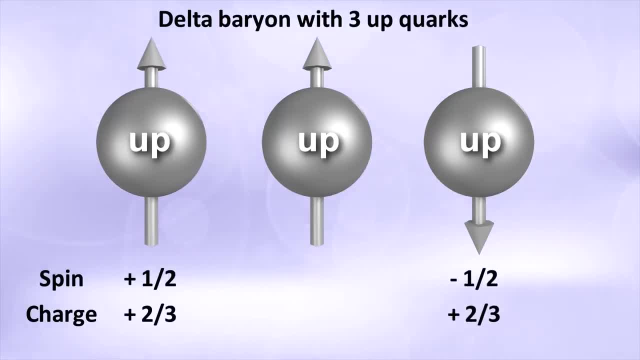 half one, that is minus one half. but the third one would have to have either a positive one half spin or a negative one half spin. Making it identical to one half spin the other up quarks. This would violate the Pauli exclusion principle. So how is it that a delta? 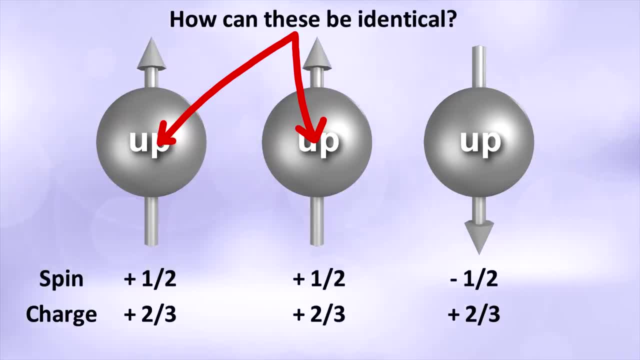 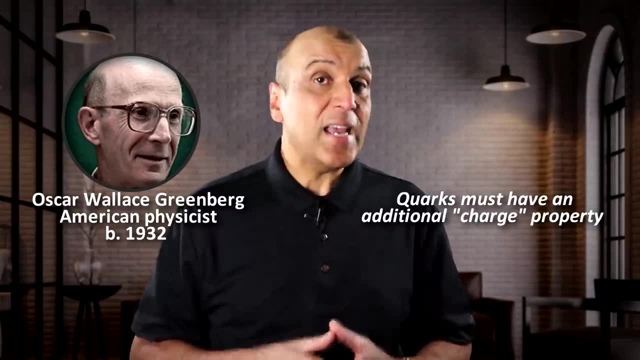 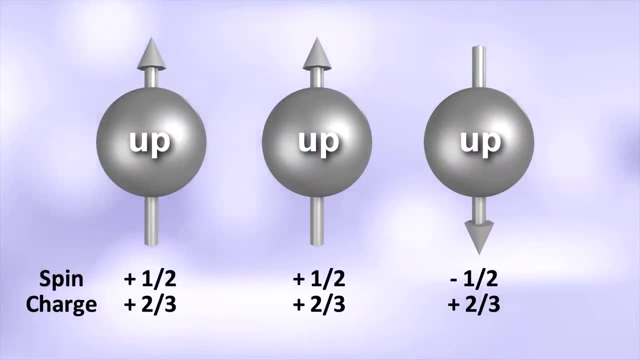 particle can exist with three of the same types of quarks. This was quite a conundrum. In 1964, American physicist Wally Greenberg proposed that quarks must have an additional property that Gell-Mann and Zweig did not consider. This additional property is now called color. 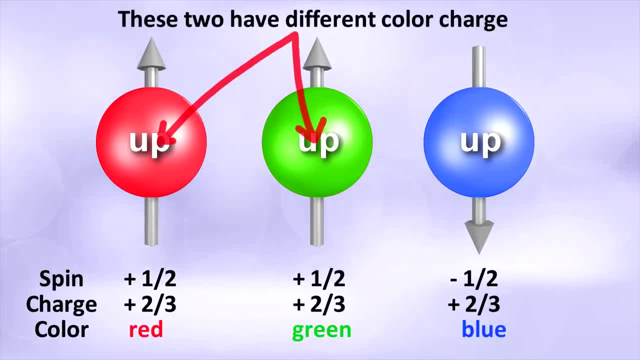 This has nothing to do with the color that you can see with your eyes. It's a metaphor for a kind of charge, a color charge. So if this was the case, the three similar up quarks would not be identical because they would have different. 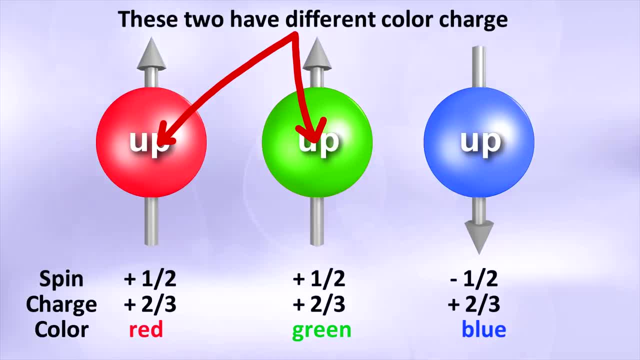 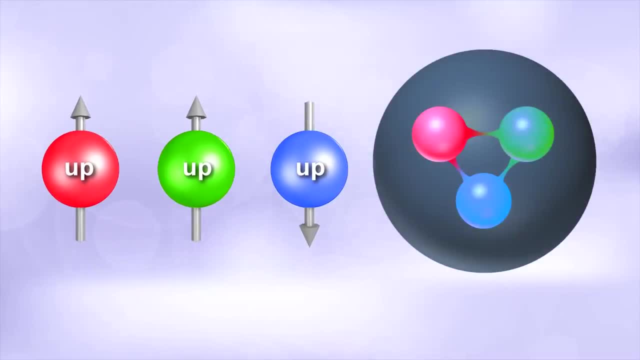 color charges and thus they would not violate the Pauli exclusion principle. They could exist in the same place making up the delta particle. There are three kinds of color: red, green and blue. The color metaphor is apt because in order to get a neutral charge, you have to combine colors, Just like when you combine. 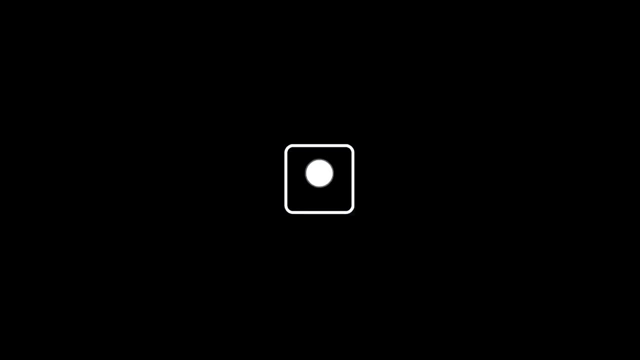 the visible and the invisible colors- red, green and blue- you get a neutral white. This is similar to the way electric charge is conserved in QED. If you have two negatively charged particles coming in, you must have two negatively charged particles coming out In QCD color must be conserved. 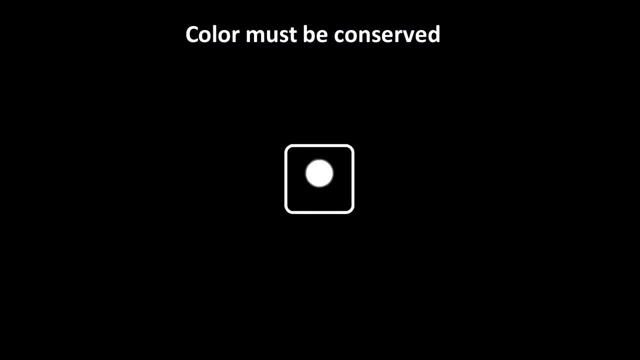 That is all. the colors must combine to get a neutral white. This means that any particles containing color charges must combine with others to form a neutral color. Three quarks, if they form a particle, must be red, green and blue to be neutral. They can't be red, red and blue. 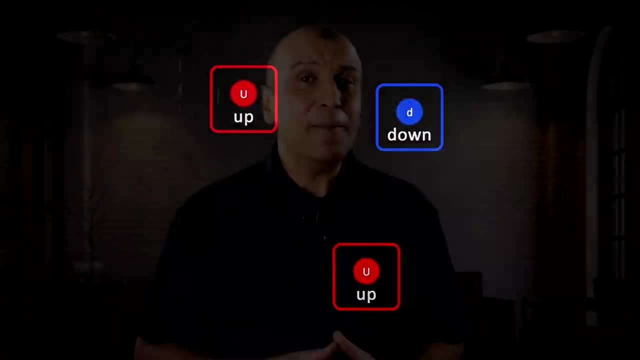 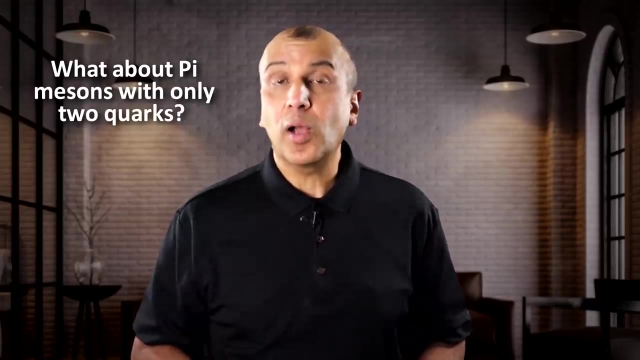 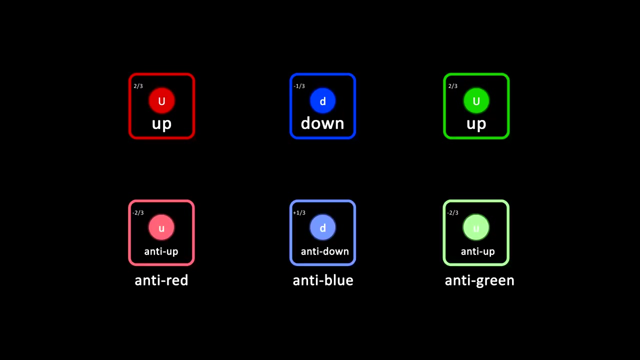 for example, or blue, blue and green. Now you might say: what about the pi-maison, which is only composed of two quarks? How do two quarks form a neutral color? Well, it turns out that they are anti-colors, called anti-red, anti-green and anti-blue. 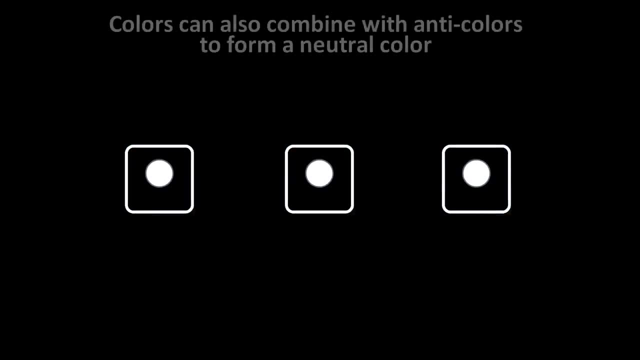 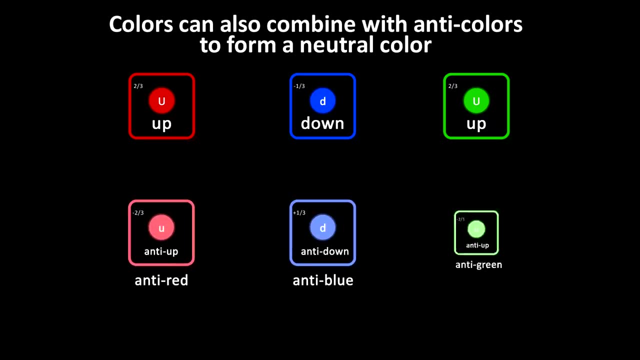 And when color-anti-color charges combine, they also form a neutral color charge. So a pi-maison, for example, can have a combination of a green color-charged up quark and an anti-green colored up quark. Such a particle would have a neutral color charge. 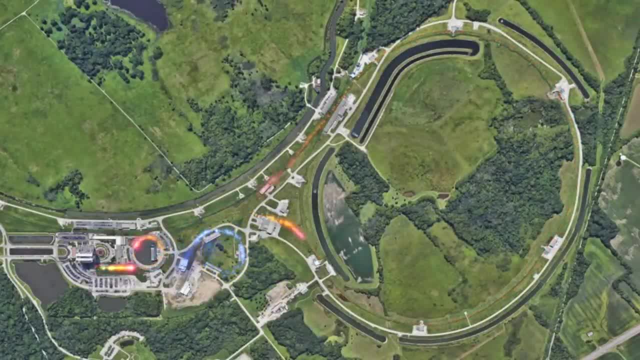 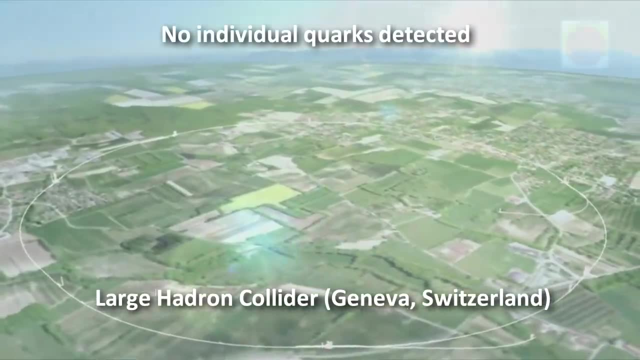 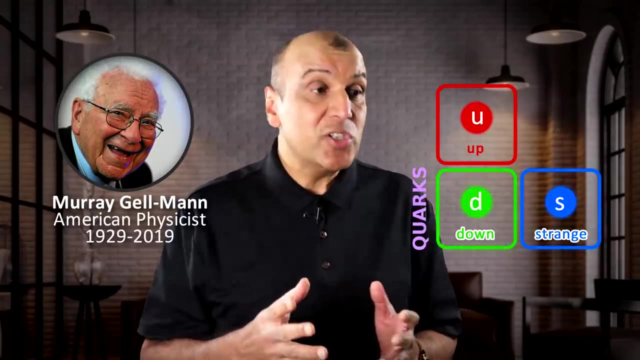 and a neutral electrical charge. Now, while the predicted quark combinations have been detected in particle accelerators, providing credence to the quark theory model, the problem was that no one had ever detected a quark by itself, And because of this, Gelman even thought that maybe his theory was just a mathematical. 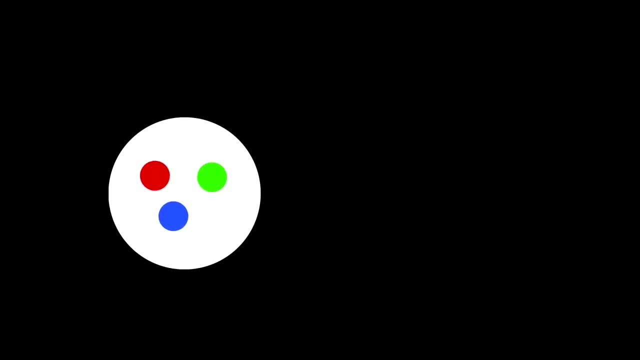 construct and that quarks were not actually real particles. Scientists came up with an idea called quark confinement to explain that quarks must be confined somehow to within the nucleon, which is another name for protons and neutrons. This implied that there must be something strongly holding these quarks together within the nucleon. 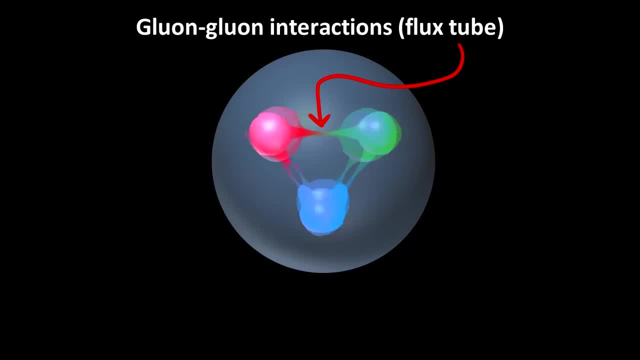 Some new particle must exist to confer this attractive force for quarks. This particle was called a gluon, because it acts like the glue that keeps quarks together. How do these gluons work? Well, first of all they form a neutral color charge, and then they form a neutral color charge. 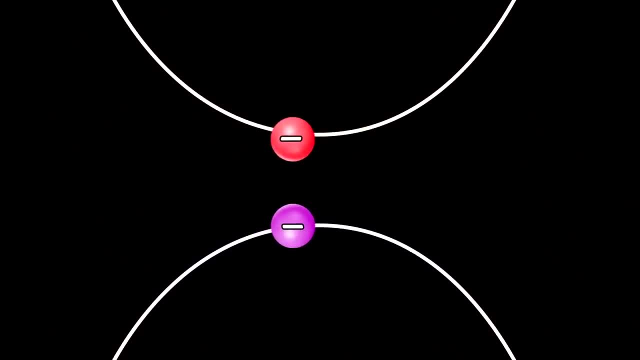 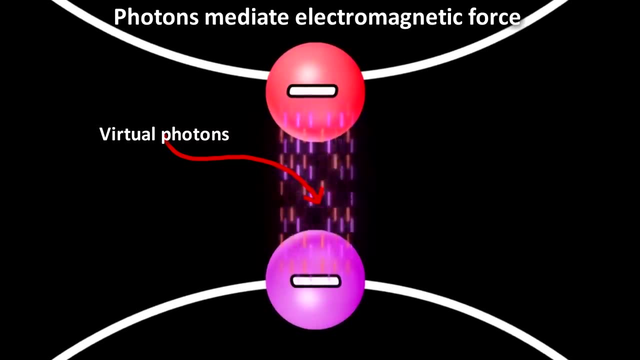 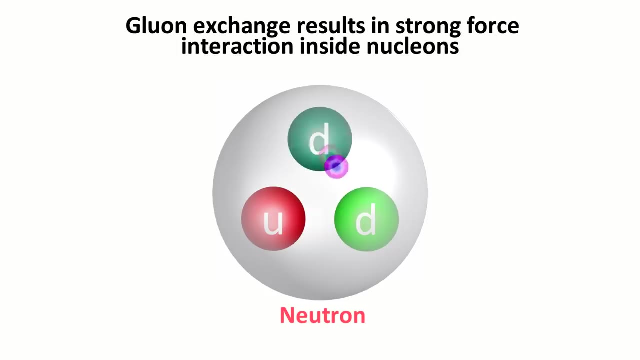 This is the crux of quantum chromodynamics, Similar to the way QED, or quantum electrodynamics, deals with electric charges and photons as the mediating particle for the electromagnetic force. QCD deals with color charges and the mediating particle for it, called gluons. 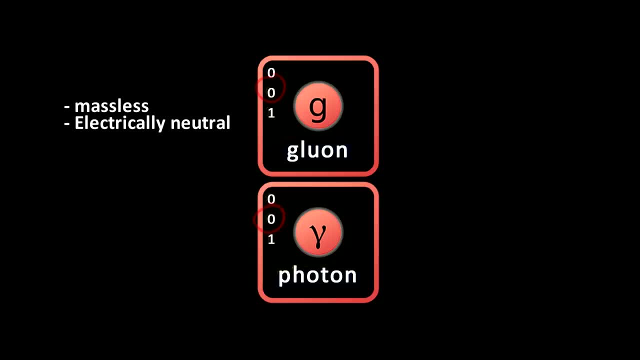 Like the photon, gluons are massless. The difference is that the photons are electrically neutral, so while they transmit the electromagnetic force, they do not experience it, nor do they interact with each other. The gluon, on the other hand, not only transmits the strong force, but also has a color charge itself. 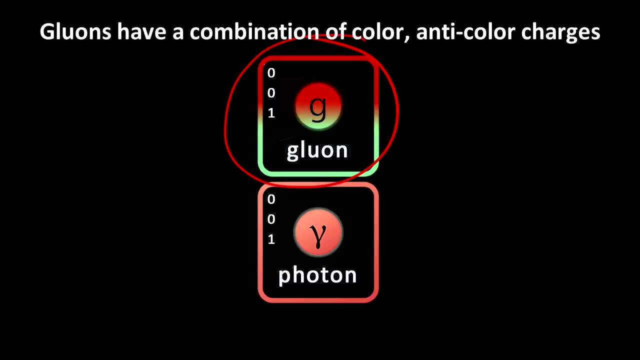 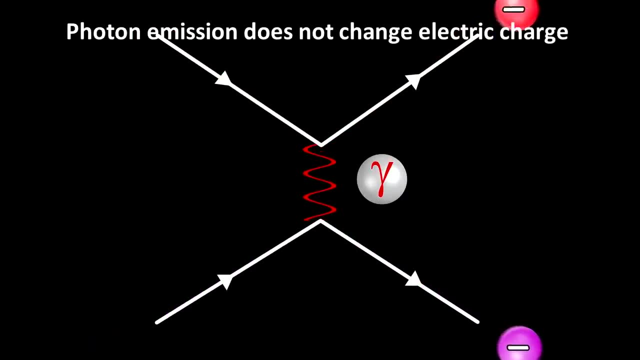 So it experiences the strong force, meaning gluons interact with other gluons. This has other implications as well. In QED, when an electron emits a photon, it remains negatively charged, But when, for example, a red quark emits a gluon, since the gluon will carry. 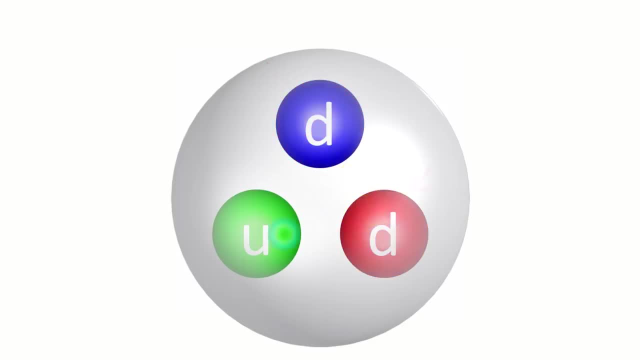 the red color, it will result in a change of color of the quark to green or blue. The colors are constantly changing within the nucleons as the gluons are being emitted and absorbed all the time. As you pull two quarks apart, the strong force acts like a rubber band. 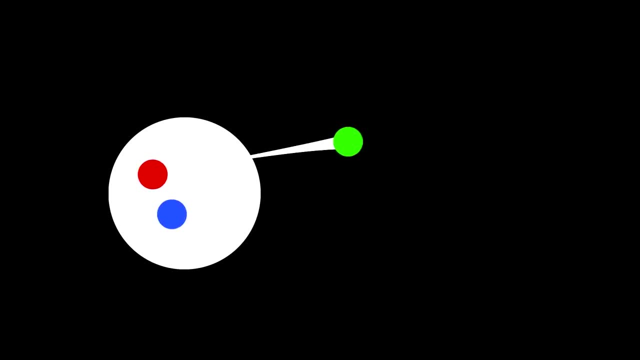 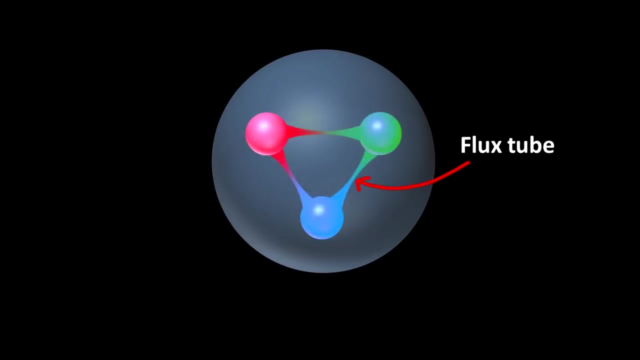 The further you pull them apart, the more and more energy it takes. This tends to pull the quark back inside the proton or neutron. These gluon-gluon interactions constrain the color fields to string-like objects called flux tubes, which exert constant force when stretched. But if a quark is pulled with enough, 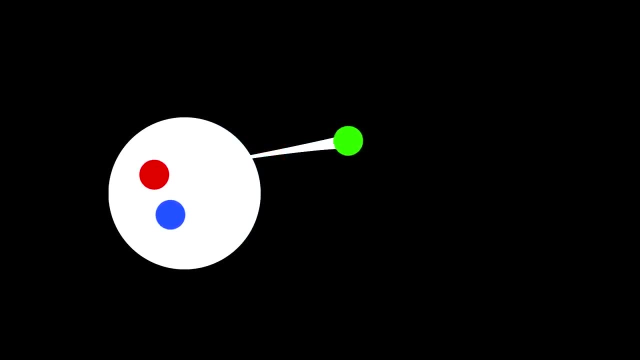 energy it pulls away until the flux tube breaks Like a rubber band. if you try to pull it apart it becomes increasingly difficult. But if you put in enough energy the flux tube breaks, just like a rubber band breaks. But the energy expended in pulling the quarks apart, 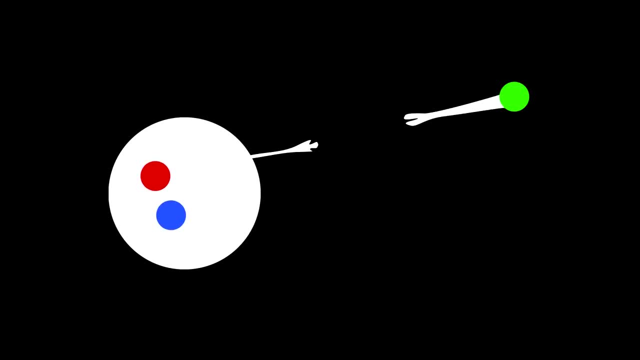 results in a surprising outcome. At the instant the quark is pulled free from the nucleon, a new quark is formed in its place, And the quark that just pulled free will, at the same instance, be coupled with another newly formed, anti-quark. 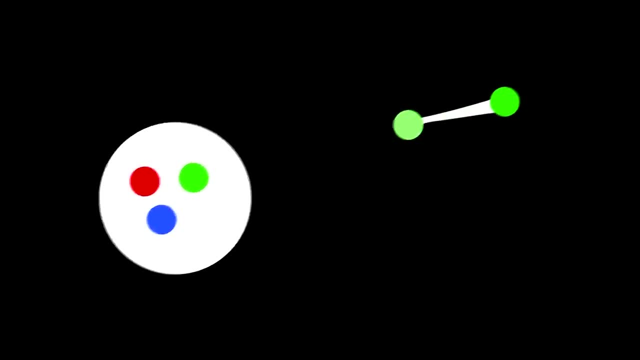 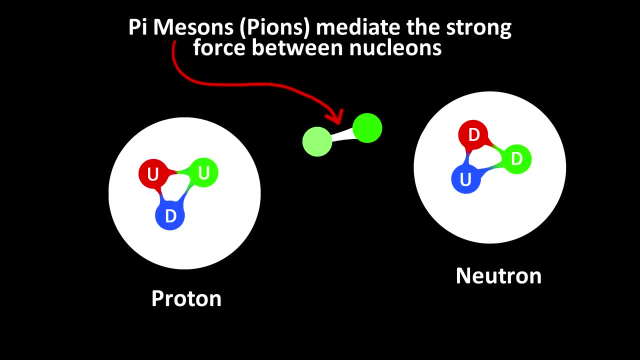 This quark-anti-quark pair is a meson. More and more mesons can be created depending on the energy available. It is these mesons that mediate the remnant of the strong force which binds protons to other protons and neutrons. In other words, residual pi mesons cause attraction. 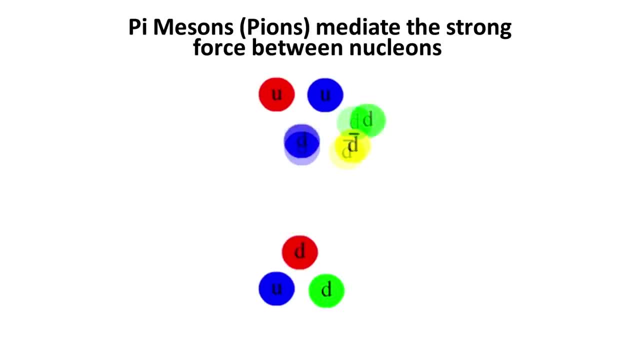 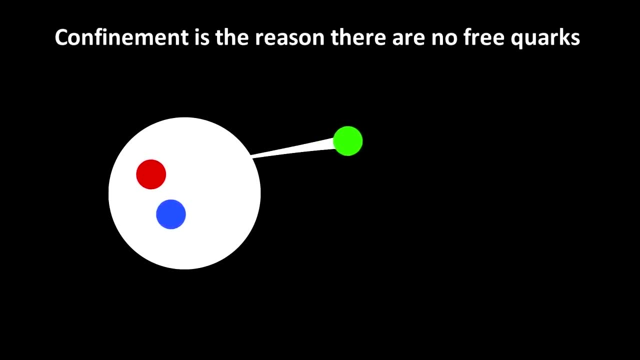 between neutrons and protons. The reason why it is so hard to pull the quark out of the proton is that you must use enough energy in the process to create at least two new quarks. This is called confinement, and it is the reason quarks remain bound to the nucleon. 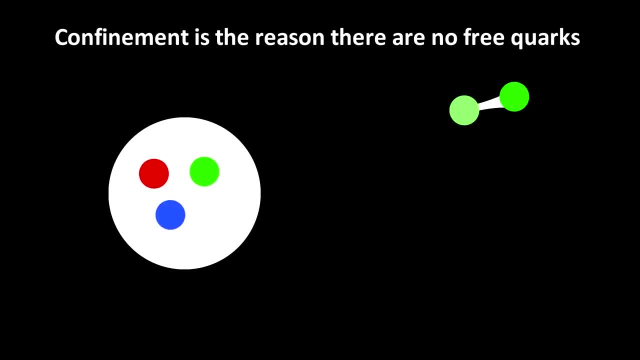 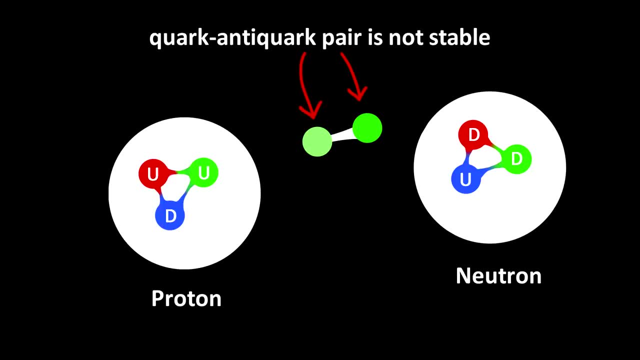 This is also the reason why no free quarks have ever been detected. Note also that the mesons are a form of matter-antimatter particle which do not last long and are unstable. The longest lasts for only a few hundreds of a microsecond. This effectively limits. 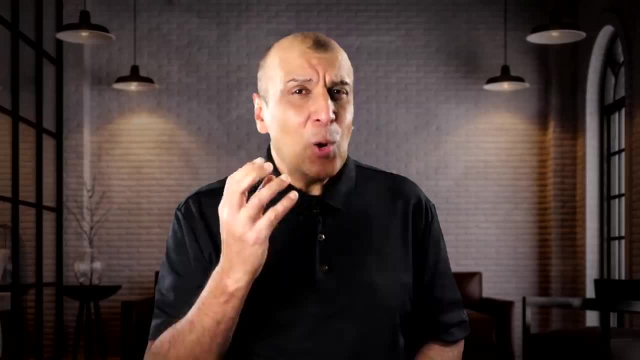 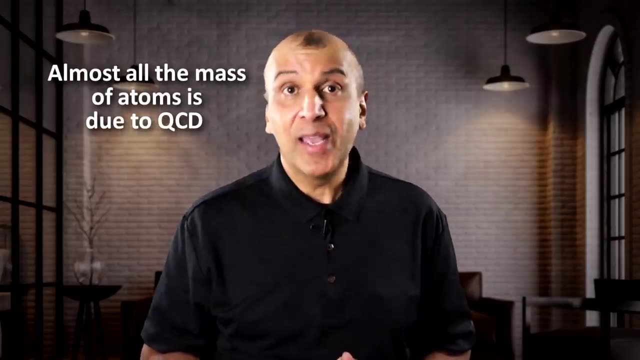 their range to within less than the diameter of a proton. One of the most important aspects of the strong nuclear force is that almost all the mass is due to QCD, not the Higgs field. How is this possible? Let's take a look at the proton, for example. A proton consists: 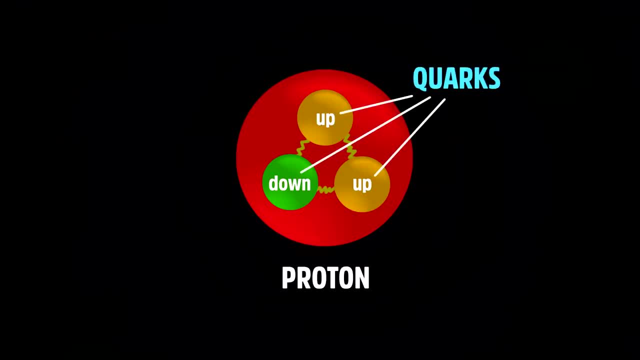 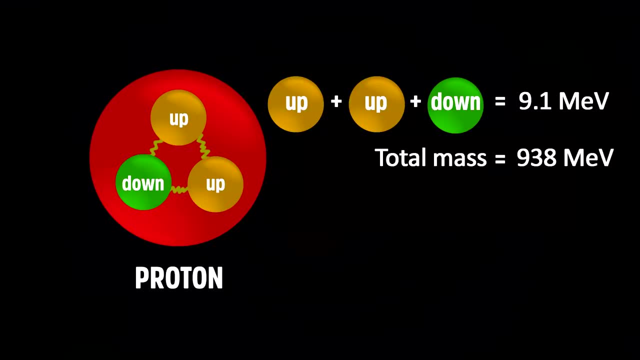 of two up quarks and a down quark. The Higgs field is responsible for giving rest mass to quarks. In this case, the combined mass of two up quarks and a down quark is 9.1 MeV, But the measured mass of the proton is 938 MeV, So it weighs about 100 times more than. 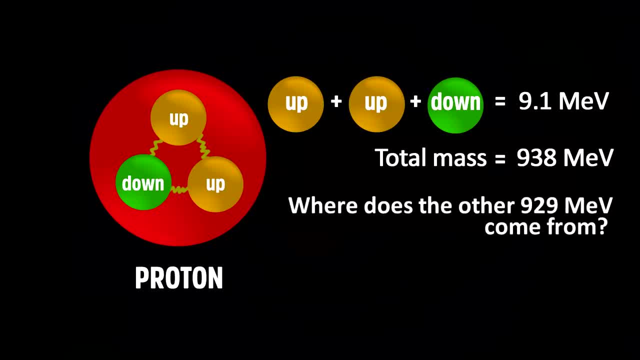 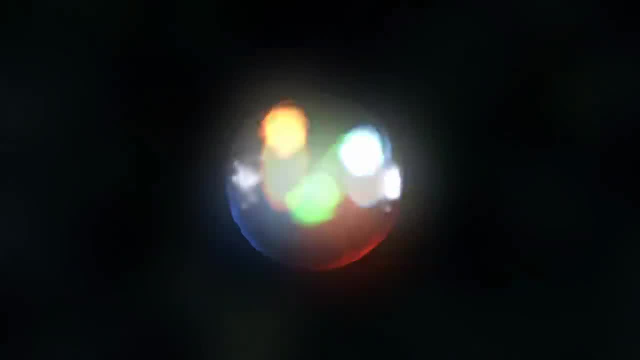 its constituent particles. Where does this extra mass come from? Well, you have to remember that quarks and gluons are moving very fast in a very tight space. To keep that much energy in such a small volume requires a lot of binding energy.